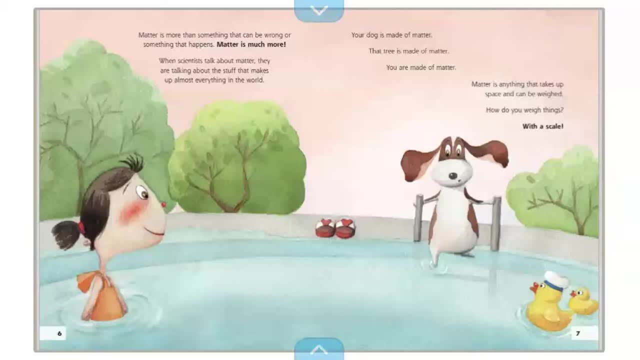 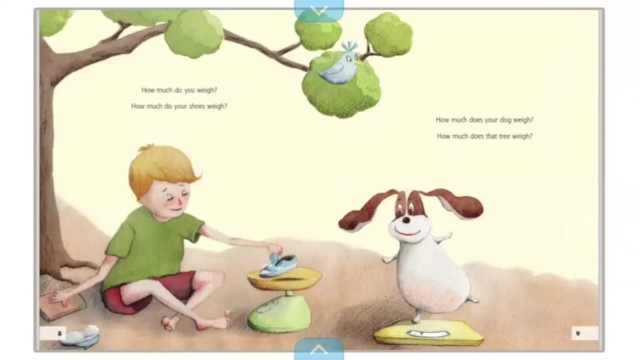 is made of matter. That tree is made of matter. You are made of matter. Matter is anything that takes up space and can be weighed. How do you weigh things? With a scale? How much do you weigh? How much do your shoes weigh? How much does your dog weigh? How much? 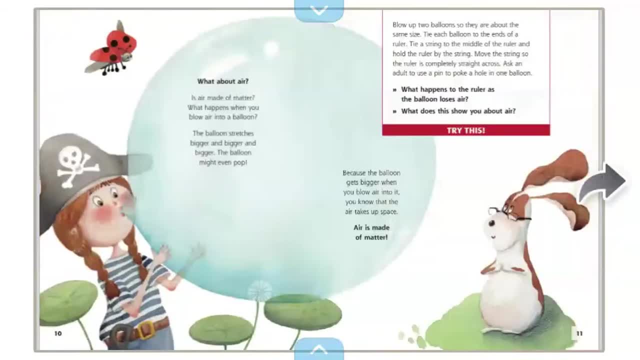 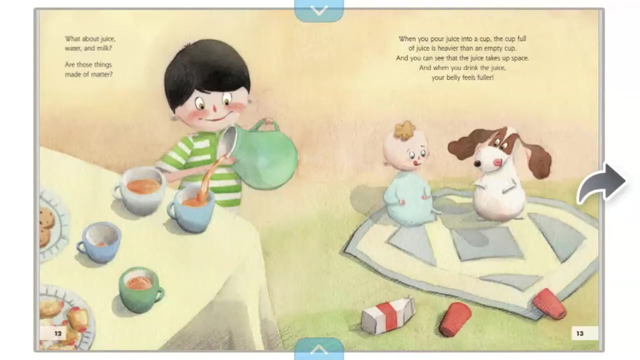 does that tree weigh? What about air? Is air made of matter? What happens when you blow air into a balloon? The balloon stretches bigger and bigger and bigger. The balloon might even pop, Because the balloon gets bigger when you blow air into it. you know that the air takes up space. Air is made of matter. 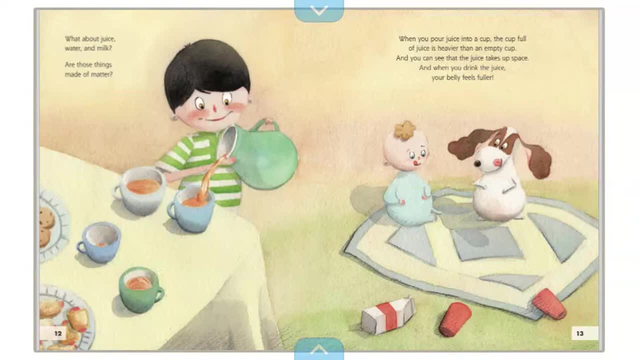 What about juice, water and milk? Are those things made of matter? When you pour juice into a cup, the cup full of juice is heavier than an empty cup And you can see that the juice takes up space. And when you drink the juice, your belly. 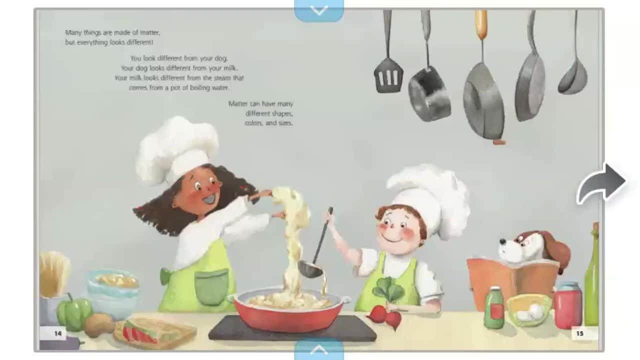 feels fuller. Many things are made of matter, But everything looks different. You look different from your dog. Your dog looks different from your milk. Your milk looks different from the steam that comes from a pot of boiling water. Matter can have many different shapes, colors and sizes. 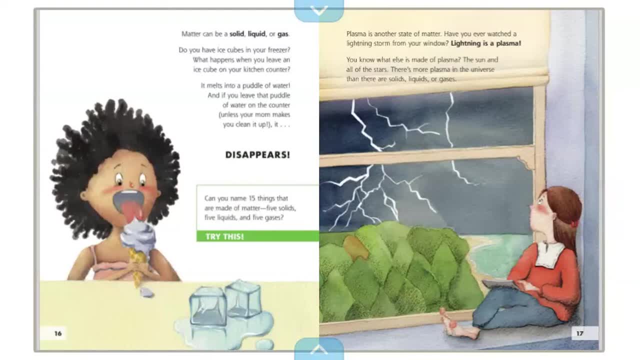 Matter can be solid, liquid or gas. Do you have ice cubes in your freezer? What happens when you leave an ice cube on your kitchen counter? It melts into a puddle of water. If you leave that puddle of water on the counter, unless your mom makes you clean it up, it. 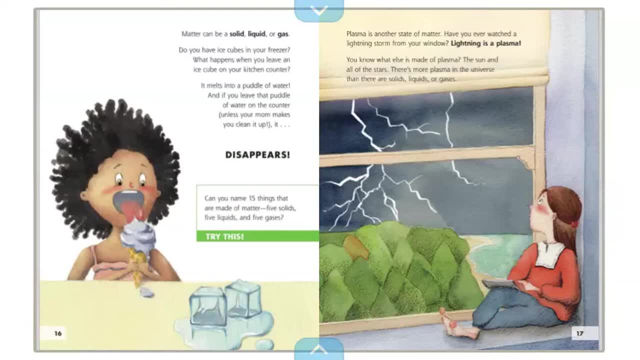 disappears. Can you name fifteen things that are made of matter? Five, six, seven, eight, five solids, five liquids and five gases? Try this. Plasma is another state of matter. Have you ever watched a lightning storm from your window?